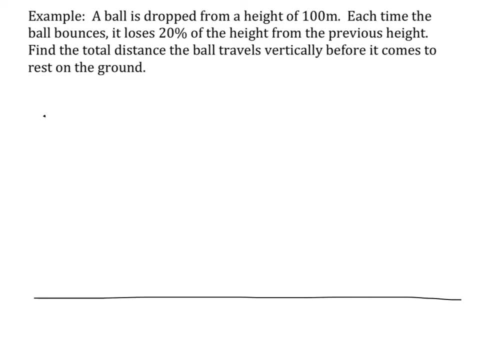 and there's, There's, you know, maybe a building here. We don't even need to draw the building, but the idea is, the ball starts out up here and sort of falls down 100 meters. We then know that each time the ball bounces, it loses 20% of the height from the previous height. 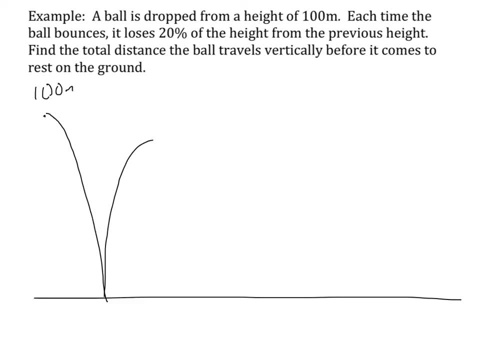 So that means that when this ball bounces back up, it's sort of going to come back up, you know, 80 meters and then it's going to go back down another 80 meters. So in some sense that bounce there will have represented 2 times 80.. 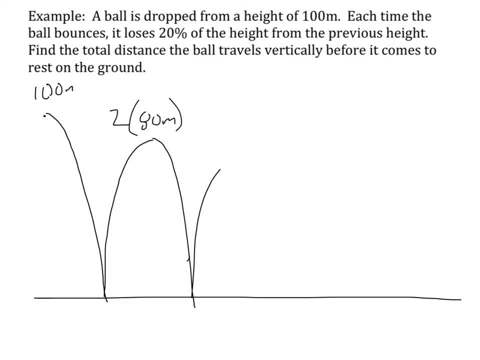 Right On the next one. you know we can sort of see what's going to happen here, right, When it hits the ground it's going to bounce back up. This time it's only going to bounce back up 80% of the 80 meters that it fell the first time. 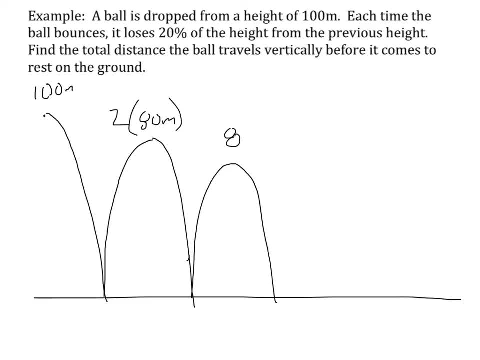 So there's sort of this sense of like: all right, well, you know, I'm going to have whatever. 80 is times 0.8, and that will happen twice. right, We could even talk about the next bounce, right? 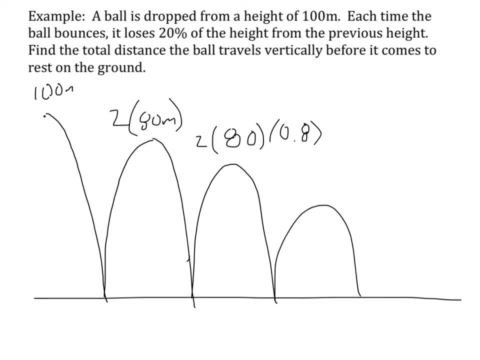 On this one it will be whatever this height was, but only 80% of that. So you almost have this sense of like. well, there was 80, and on the previous one it only went 80% of that. 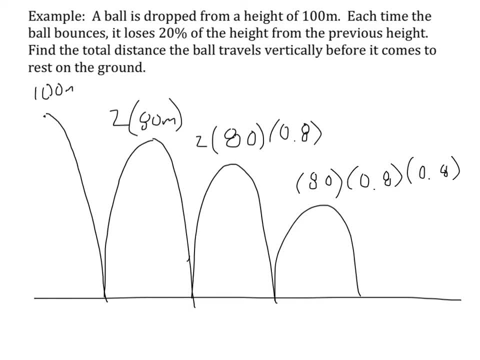 and on this one it's actually only going to go 80% of that, and because we're going both up and down, we'll have 2 of that as well, And so what I hope you guys see here is that this is effectively the setup for an infinite geometric series. 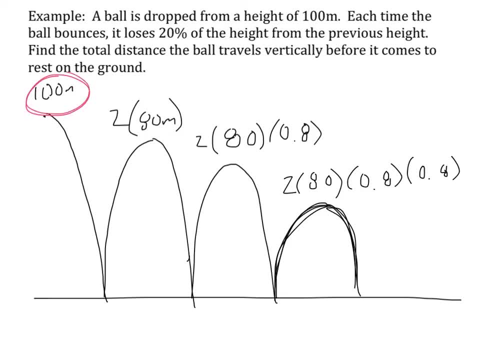 Just like we saw in the repeating decimal, this is sort of like an irregular initial term. There was this initial 100 meter bounce, but from that point on you have this initial bounce, you have 80% of that initial bounce, you have 80% of that second bounce. 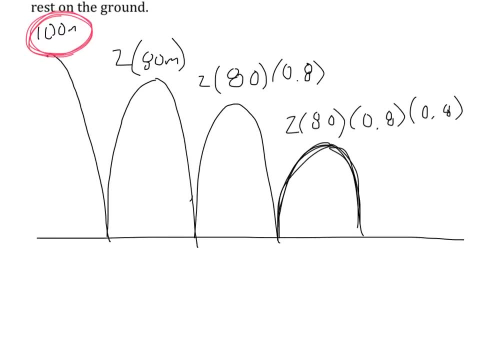 We can sort of see here that there's a very clear first term and there's a very clear common ratio, right? It seems to me that my first term in this problem, the first term of the geometric portion of this part, is the 2 times 80, right? 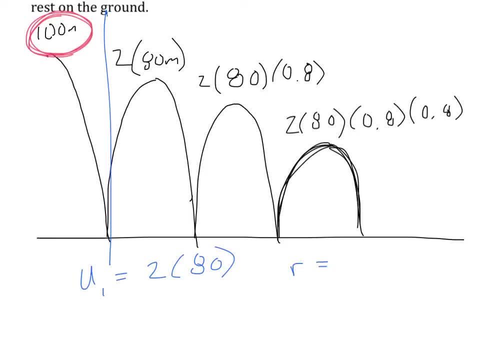 What's the common ratio? What's happening each successive time? Each successive time, we're bouncing only 80% as high. So my common ratio will be 0.8, which we could write as 4.. So it's 1 minus 4 fifths right. 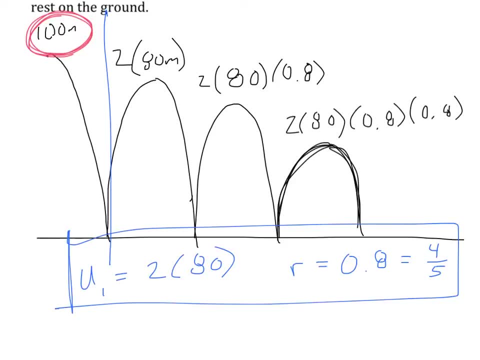 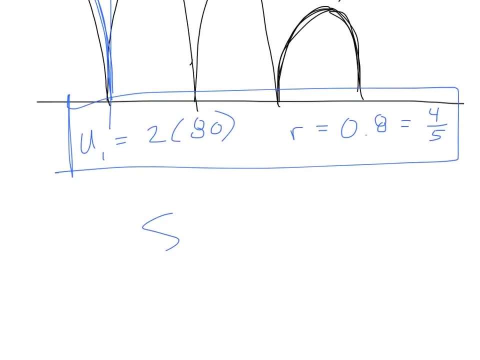 And the idea is, we will figure out what this is and then we'll add on the initial 100 meter fall that we had. So we can use our formula for this. We can say that S will be the first term, which is 160,. 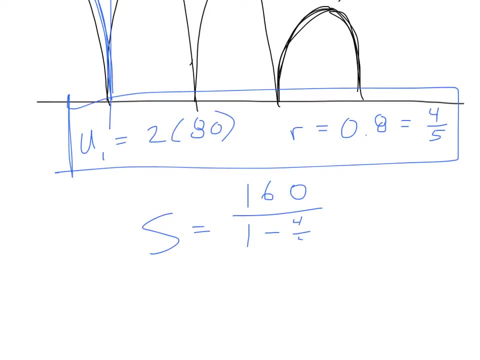 over 1 minus the common ratio, which is 4 fifths. Be careful right there. I actually just did this wrong in the video and had to rerecord it. The previous side: I just put the 4 fifths in the denominator. it's 1 minus 4 fifths. 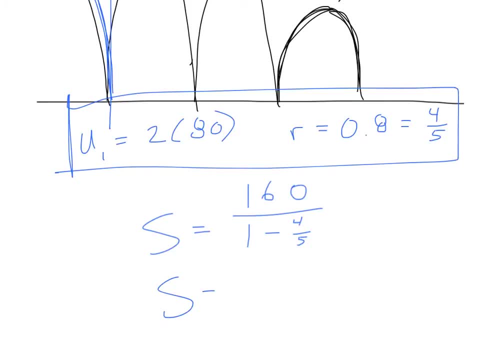 So don't forget that. that's how the formula works, right. So S is going to be 160 over 1 fifth. So I can just multiply the numerator and the denominator, both by 5, to get rid of the 1 fifth in the denominator. 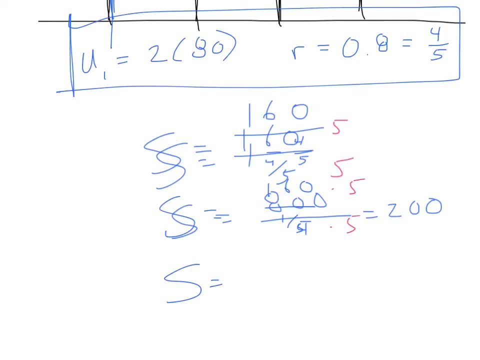 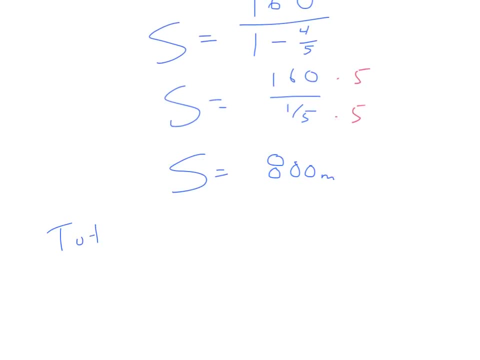 And I'll find that the total distance traveled in the geometric bouncing part of the problem is 800 meters. right, But that's not the total distance. My total distance will be the 100 initial meters that the ball fell, plus the 800.. 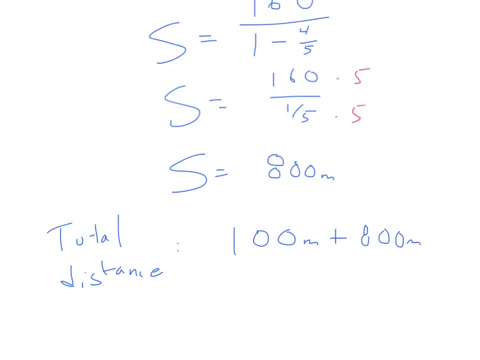 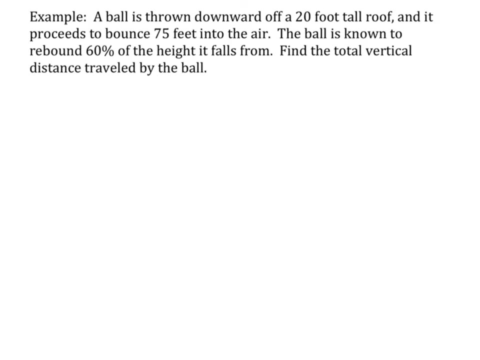 Right meters worth of geometric series bouncing part. So my total distance here is going to be 900 meters. So here we have another example of the bouncing ball problem. In this case a ball is thrown downward off a 20 foot tall roof and it proceeds to bounce. 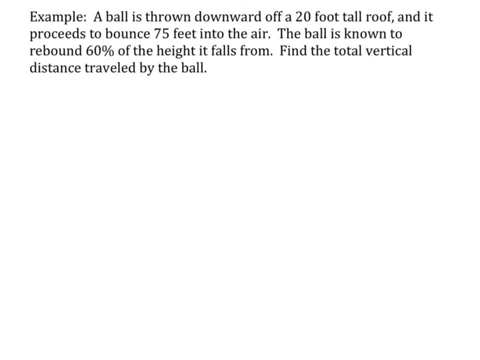 75 feet into the air. The ball is then known to rebound 60% of the height that it falls from to find the total vertical distance traveled by the ball. So I'd like you guys to pause the video, sort of see if you can set up your initial like. set up the. 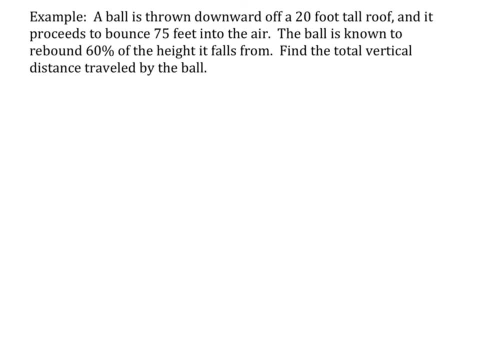 diagram for this in terms of what you're going to label and put what you're going to put where. then check back in with me and once we have that, you guys can go forward with the computation. So the idea here is that you've got the ground, there's this roof, that's, you know, 20 feet. 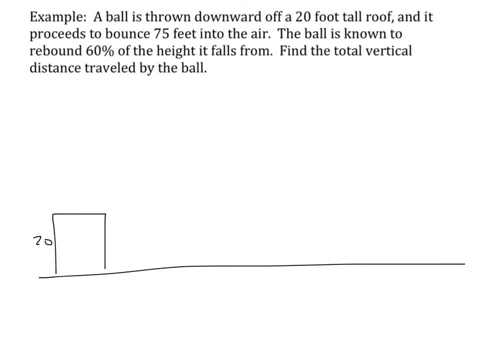 tall, alright, fine. and the ball is thrown downward off this roof and from there bounces upward 75 feet into the air. After that time, of course, it's going to fall just as far and from that point it's going to bounce. 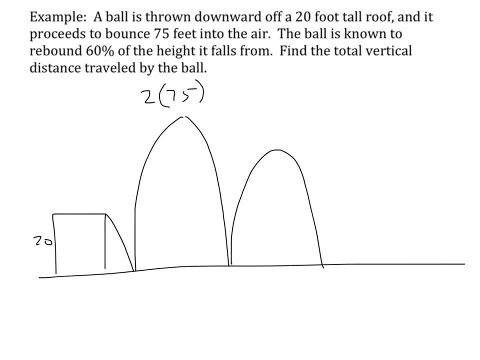 back up and back down. Think about so what's going to happen here? We're going to have that 75 foot height that it fell from. times it rebounds 60% of its height, so that's 0.6 and we're multiplying by 2 because it's going up and back down.